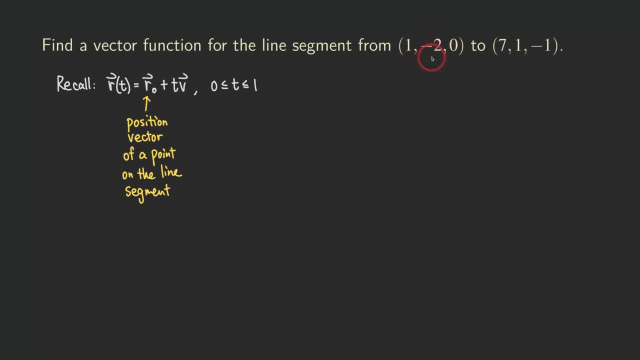 r naught to be the position vector for this point, right, In this case, call this point, this point, right here, the first point that we see in the problem. right, Because we're going from this point, right, So we call this one the initial point. And what about the? 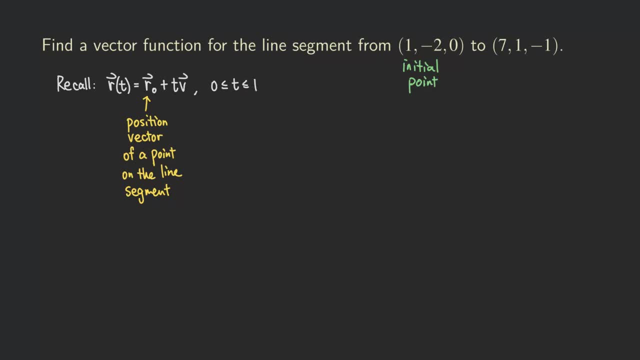 point that we get to. that would be the terminal point, right? So we can call that the terminal point of the line segment. Okay, so now one more thing that we need to specify here is that there is the V here. what is the V? the V is actually the direction vector. right, That's the vector. 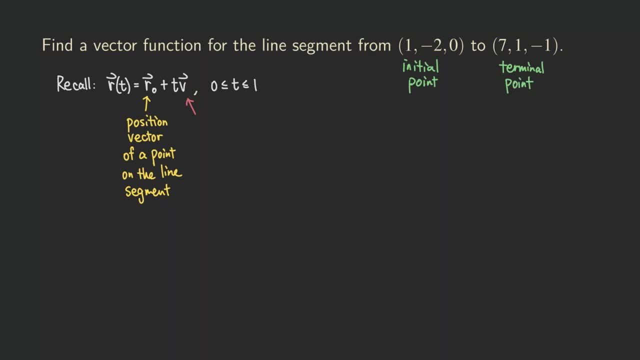 that's parallel to the line segment that we are trying to find. So this is the direction vector. Okay, so we're getting this direction vector. it can actually be found by taking the terminal point, subtracting the initial point, so that we can get a direction vector for the line segment. 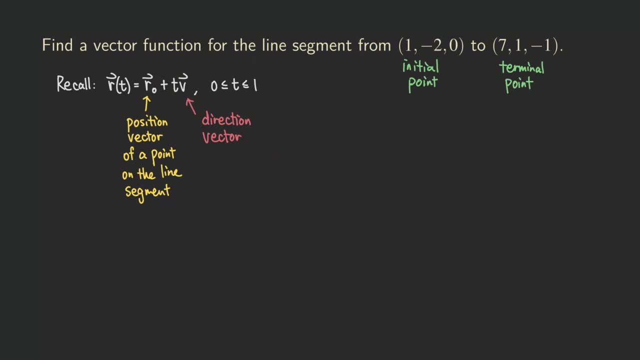 that we're trying to determine here: Okay so, okay, so there's, there's, there's, everything is ready. we are ready to actually come up with a solution, So let's do that. So first we are going to just write down, we're just going to write down the R naught. 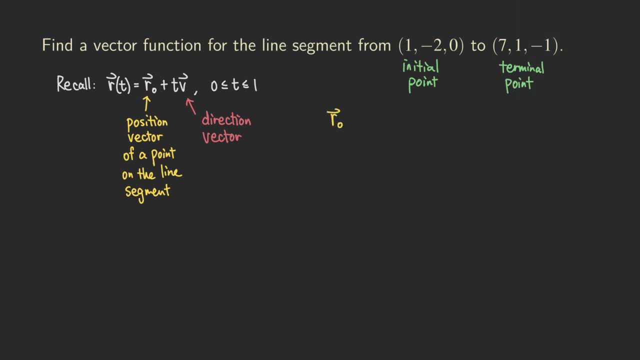 which is what is that? the R naught is actually our initial point, right. so we are going to be getting just this point right here. But remember, it's a vector, it's a position vector, So we are going to use just the x y z, x y z values for the x y z components. 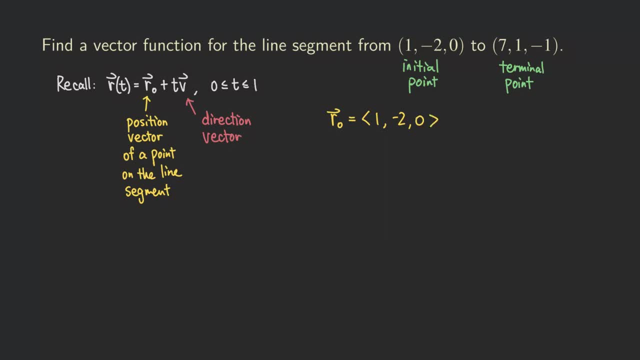 for this. And so, as you know that for position vector, the initial point is actually at the, its tail is actually at the origin, So now its head is actually the it's pointing to this point. So that's why we have one negative, two and zero. that's exactly those three values. 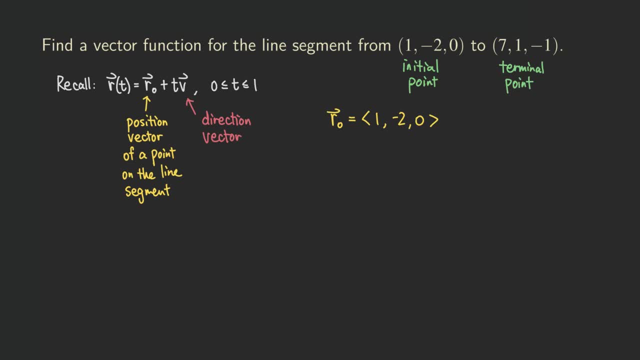 that we put here. Okay, so now the the direction vector. direction vector is going to be given by what we take: the terminal point subtracting the initial point. so it's going to be. so take the seven right, and then we minus, minus the x value of the initial point, which is one right. Okay, so we get. 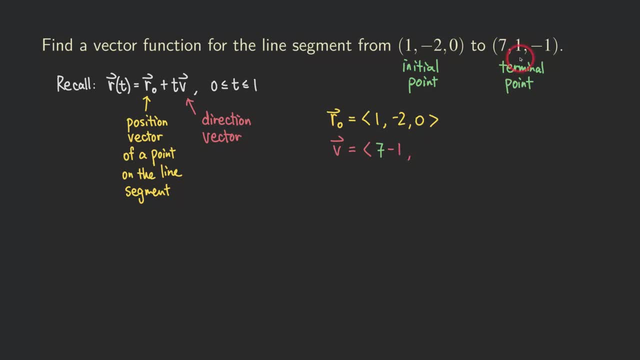 that. And then now, second component, is to take the y value of the terminal point, subtract the y value of the initial point, So we get the one here, right? Well, actually that should also be a green right, So one. and then now minus minus one, minus this legacy, two, so we get. 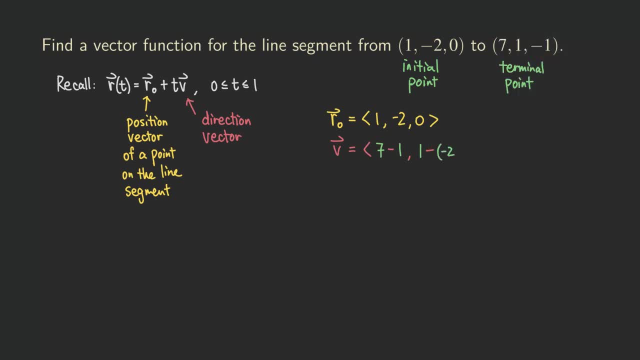 to put the legacy two here. So make sure that you don't just put the two. you got to put legacy two because this minus sign comes from constructing the direction vector. that minus sign comes from the y value at the initial point. Okay, so last component. so we are. 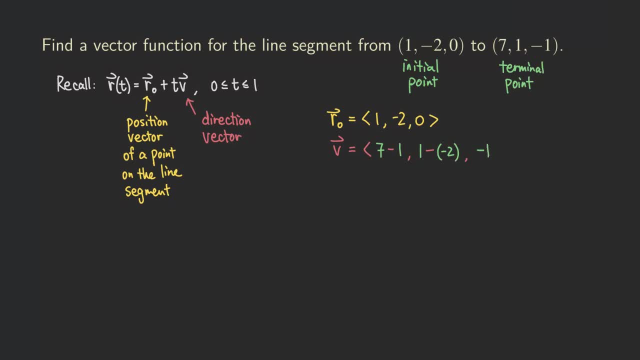 going to be getting. what is that? that's going to be minus one, right. so we are taking the Z value of the terminal point. subtract, subtract what? subtract? the zero, right, subtract the zero, okay. so now doing the calculation, we get six, we get three, we get negative one. okay, so now we have both things. 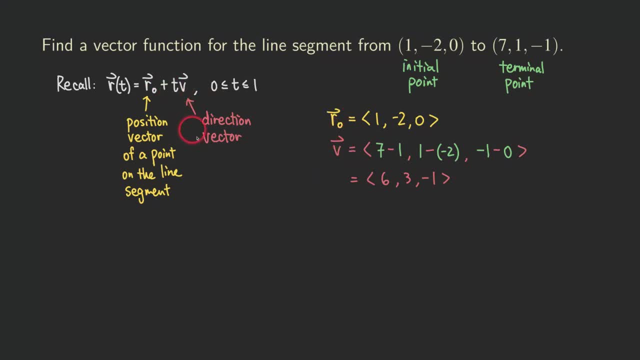 right. we have the r naught and also have the v, so we're ready to come back to the function and then just fill in everything in there. so we have r of t. that's equal to what is that? that's going to be one right, so we have. 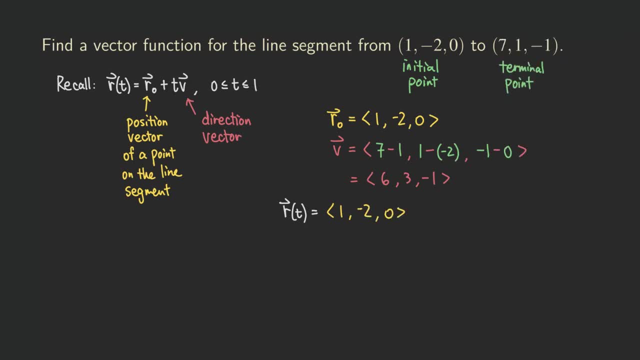 one negative, two and zero, right, and then plus t times what t times this direction vector. so six, three negative, one. okay, then let's do the calculation first. so we are going to get one negative, two, zero. distribute the t, we get six t, three t, negative t, and then just add the two vectors together, right, so we are going to be. 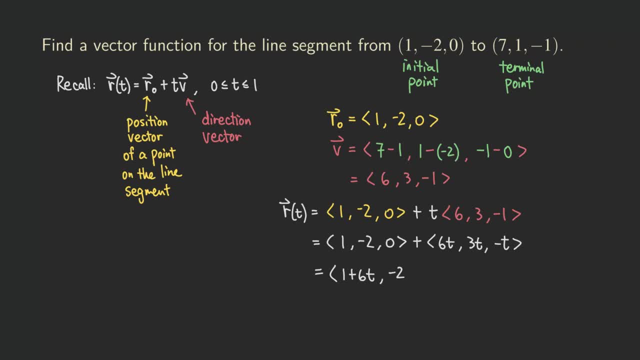 getting one plus six t, negative, two plus three t, and then zero minus t, right, so just negative t. and don't forget that we gotta put the restriction for the t right. so the domain for the t is going from zero to one, and so we can do a quick check here. so if we put it, 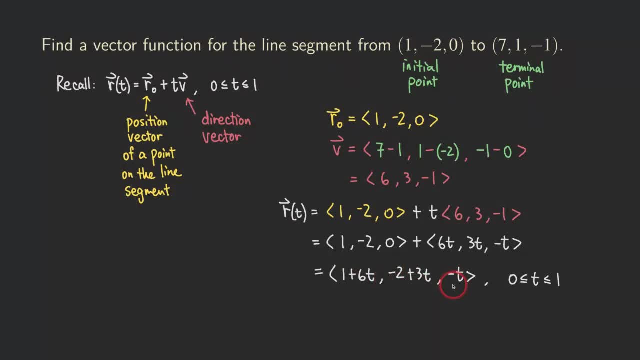 in the zero, we get one negative two, and then zero, which is exactly the initial point here. and when we put in the one, then we are going to get one plus six, which is seven. right, put in the one here, three minus two, we get one. put in the one here, we get negative one. so we are getting.